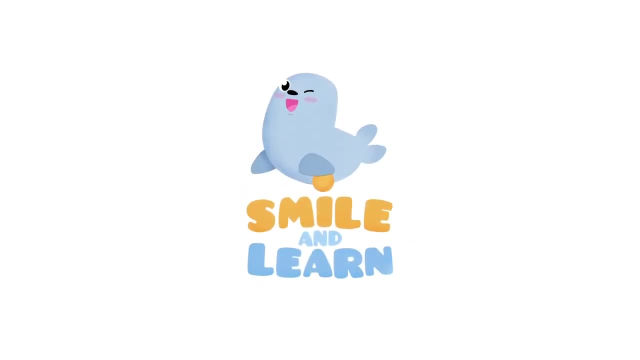 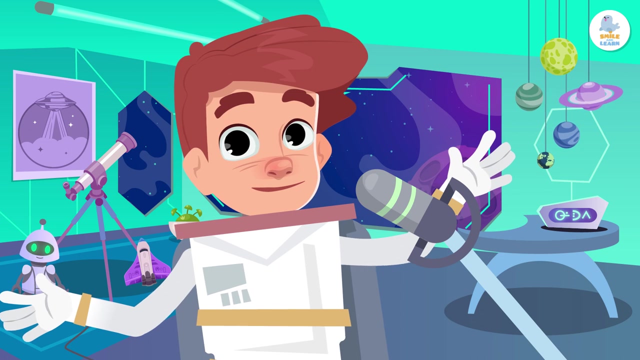 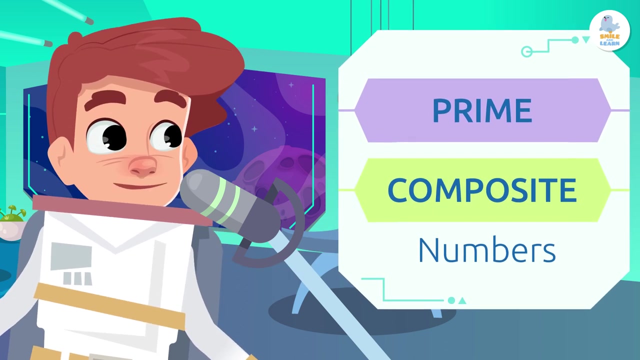 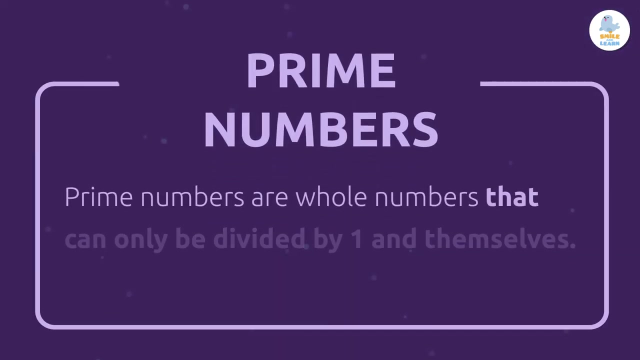 Hi friends, Today on my Space Math channel, we're going to learn what prime numbers and composite numbers are. We'll start with prime numbers. Prime numbers are whole numbers that can only be divided by one and themselves. This means that they only have two divisors. 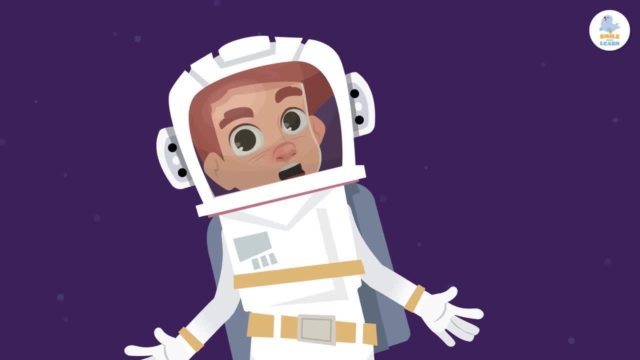 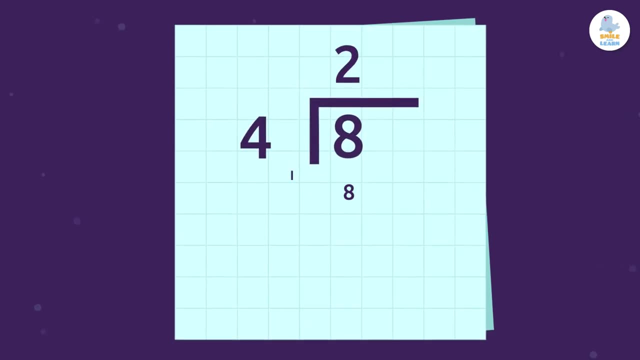 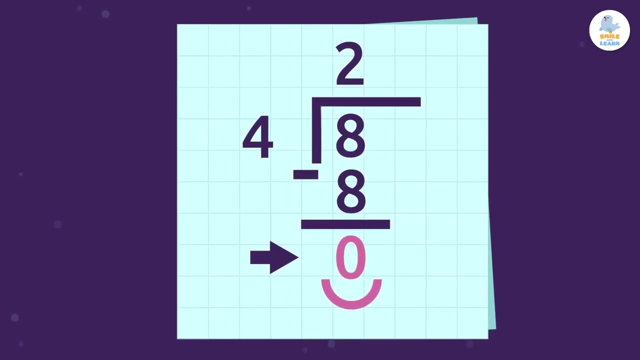 In other words, we get an exact division when we divide a prime number by itself or by the number one. Remember that a number is divisible by another only if we get an exact division, which means the remainder is zero. Let's try this with the number five. 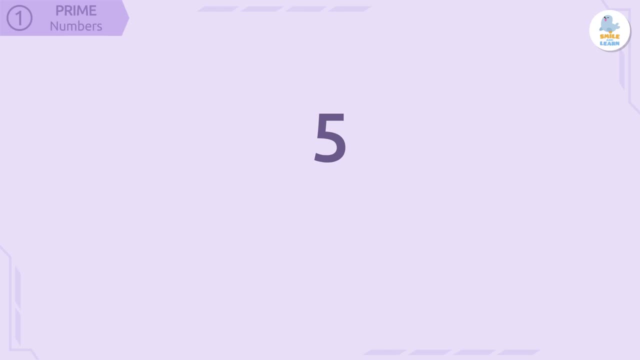 If we do five divided by one, it equals five. And now, if we do five divided by five, it equals one. But can we divide the number five by a different number and get an exact division? No, This is why the number five is a prime number. 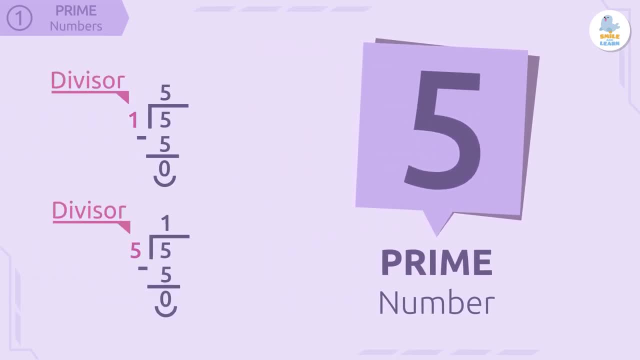 Because it only has two divisors, one and itself. Let's do another example. Now we will see if the number eleven is a prime number or not. First, let's find the divisors of eleven to check and see if it is a prime number. 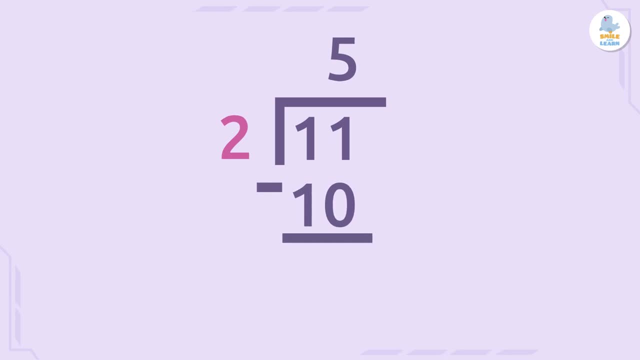 If we do eleven divided by two, we get five remainder one. This is not an exact division, so the number eleven does not have the number two as a divisor. Now we can divide the number eleven by two, But we have to check if we get an exact division when we divide eleven by all the possible numbers. 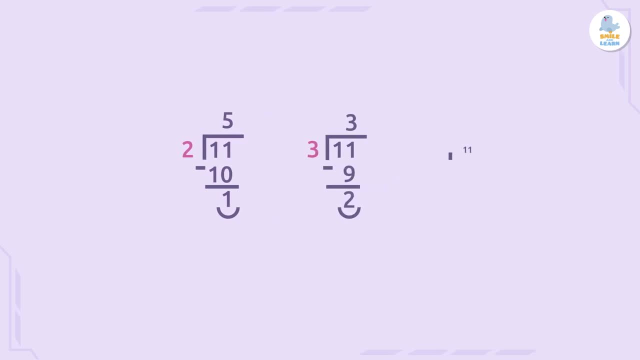 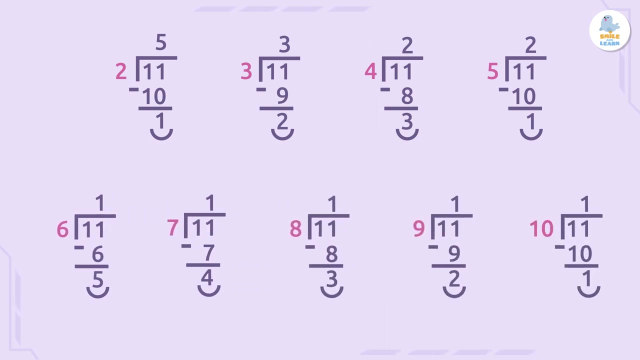 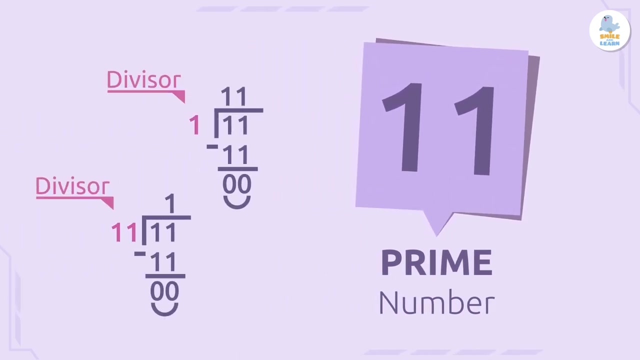 By three, By four, By five, By six, All the way up to ten. So eleven is a prime number because its divisors are only one and itself Eleven. Here is a table with the first few prime numbers. Let's take a look at it. 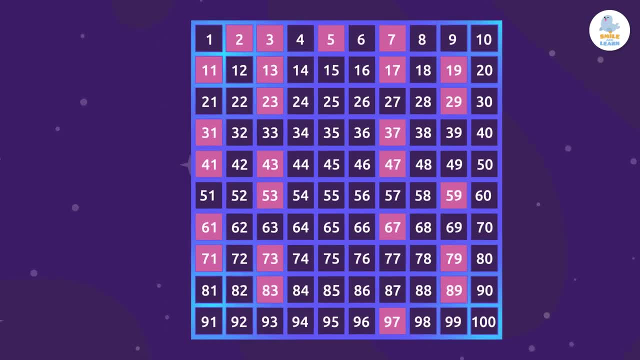 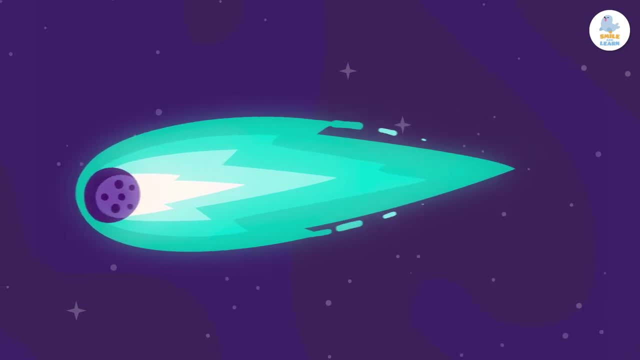 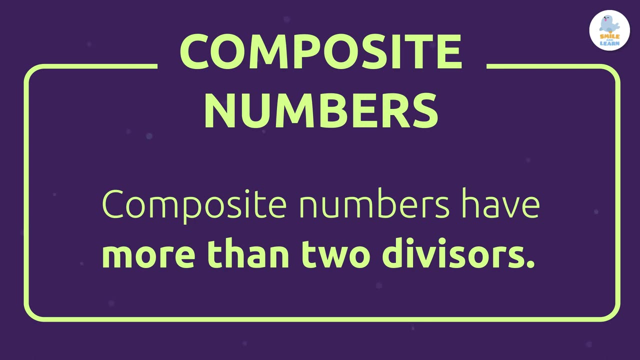 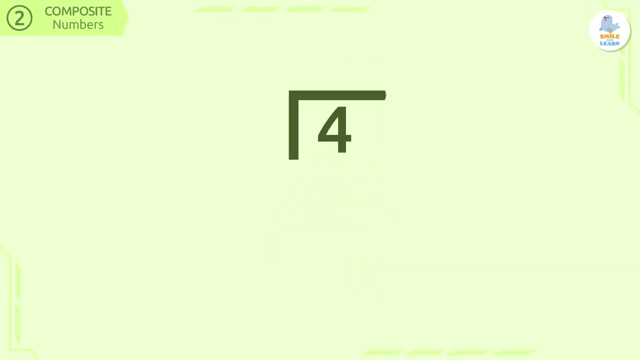 Now let's have a look at what composite numbers are. Unlike prime numbers, composite numbers have more than two divisors. Let's check this definition using number four as an example. If we divide the number four by one, we get four remainder zero as the result. 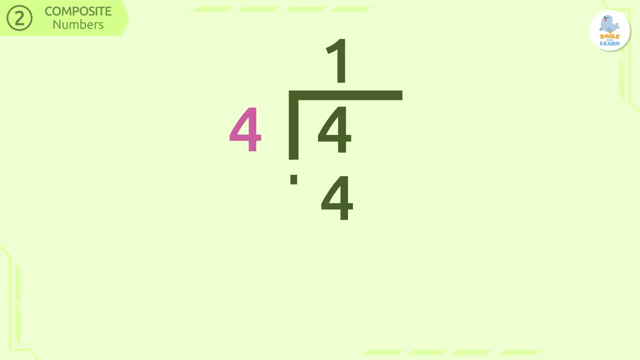 Now, let's divide the number four by four. We get one remainder zero as the result: Now we have two divisors, but does the number four have more divisors? Hmm, Let's try doing four divided by two. Very good, Here we get two remainder zero, which is an exact division. 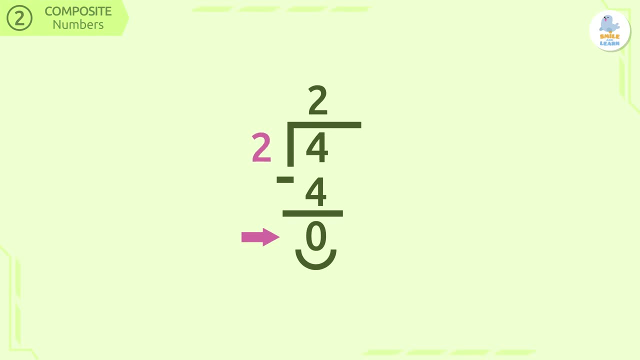 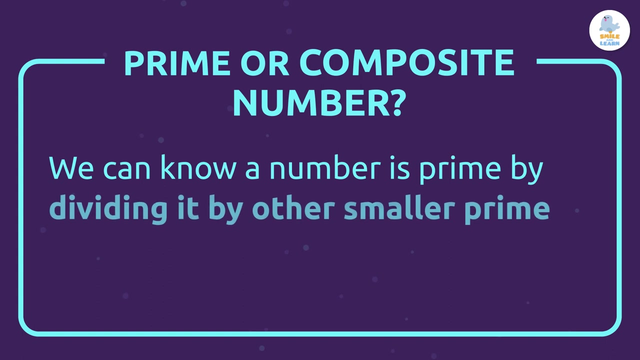 So the number two is also a divisor of four. We can see that the number four has one, two and four as its divisors. For this reason it is a composite number, as it has more than two divisors. We can know a number is prime by dividing it by other smaller prime numbers. 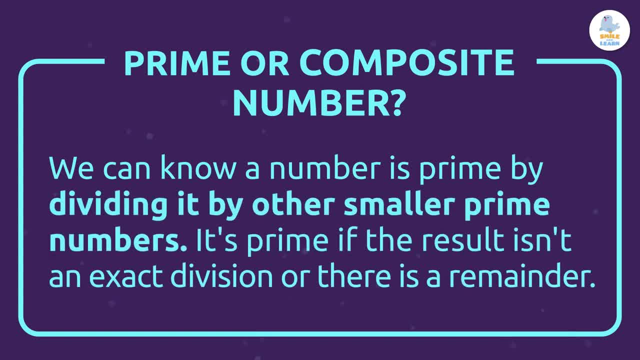 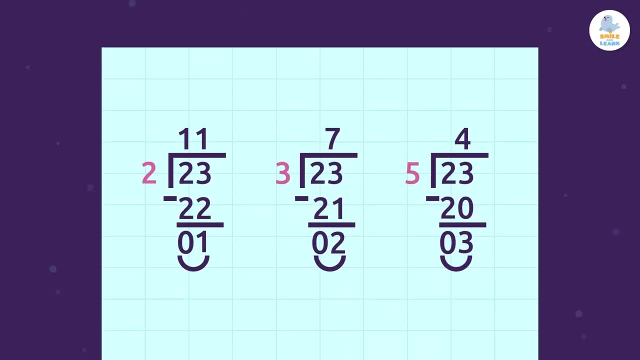 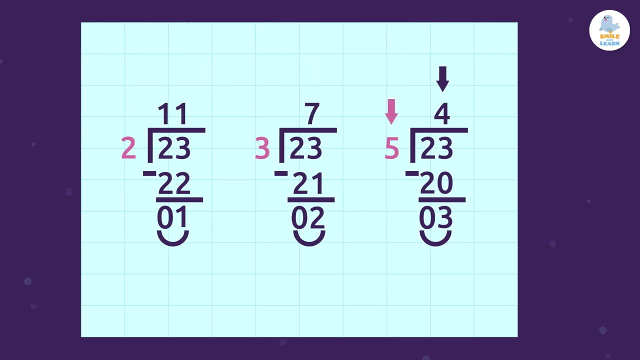 It's prime. if the result isn't an exact division or there is a remainder, We should check this by dividing the number by prime numbers smaller than it until we get a quotient that is less than the divisor. When we need to check if a larger number is prime or not, it will help us a lot to know. 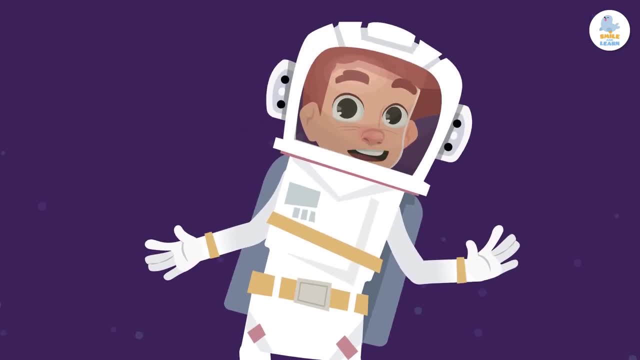 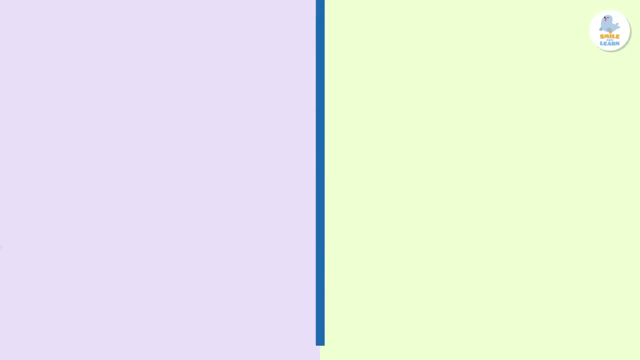 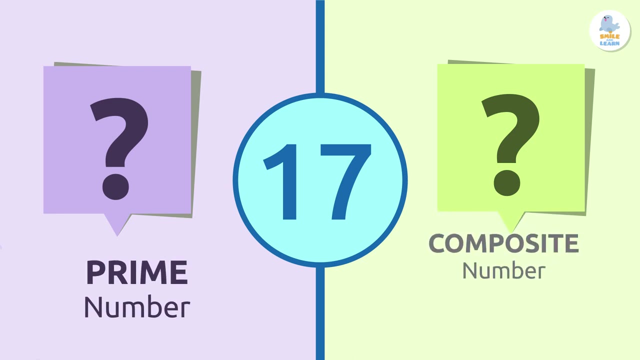 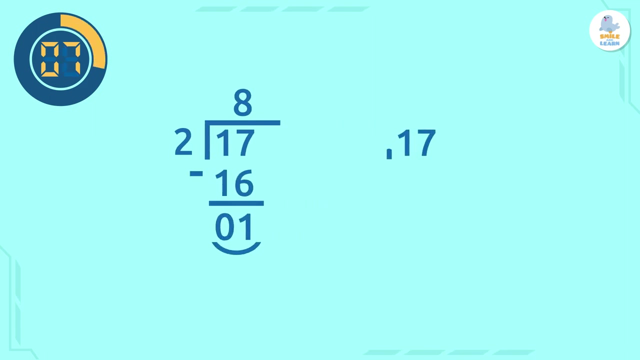 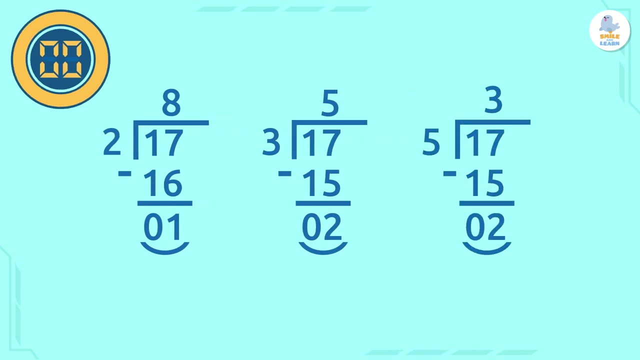 the divisibility criteria. Perhaps you can review them after watching this video. Now it's your turn. Let's see if you have understood everything correctly. Is the number 17 a prime number or a composite number? Correct, It is a prime number. 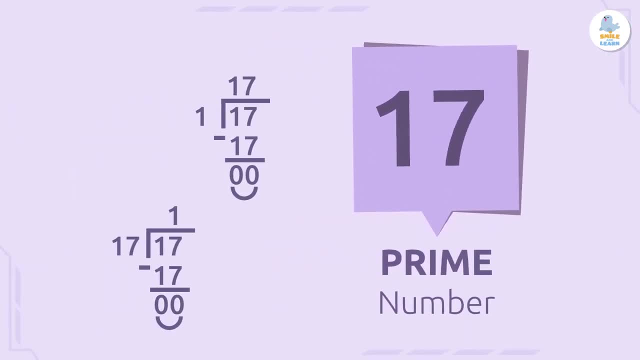 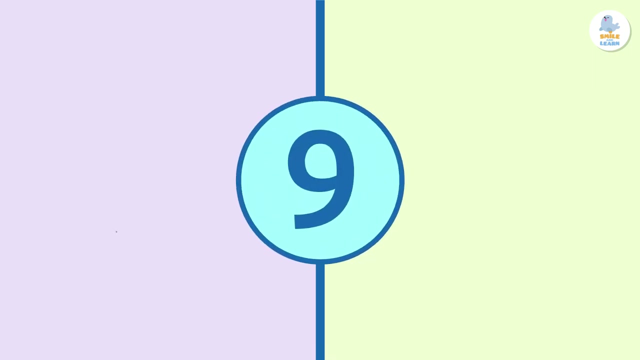 The number 17 has only two divisors: itself 17, and also the number 1. When we divide it by the smaller prime numbers, we do not get zero as a remainder in any of them. Perfect, Let's move on to the next task.